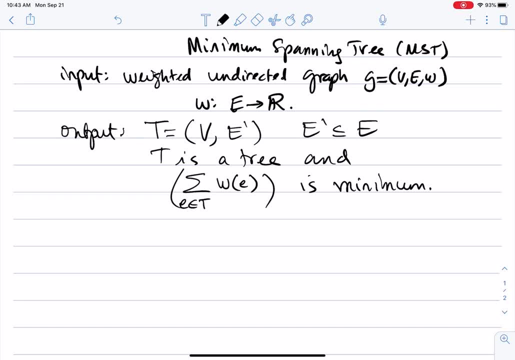 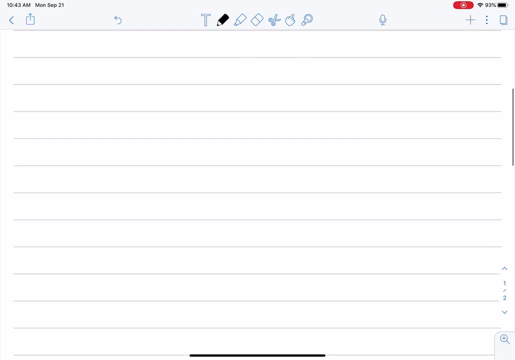 Now, this is a very, you know, very- important problem in graph theory, And this is one of the problems for which a greedy algorithm works and works. you know, it's a natural way to think about the problem, And one algorithm for this problem is known as Prim's algorithm. 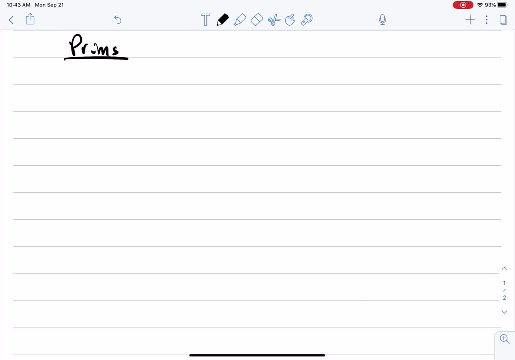 Prim's algorithm. How does Prim's algorithm work? So imagine again that 3T- the 3T that I'm looking for- has the set of edges, the set of nodes V sub T and the set of edges E sub T. okay, 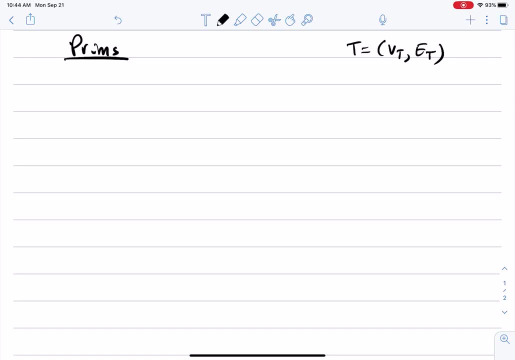 And I want to basically build them. And we start here by saying: let V sub T be some arbitrary node. okay, So this is some arbitrary node. Take whichever node, the first node you encounter in the dictionary representing the graph, you can take it, okay. 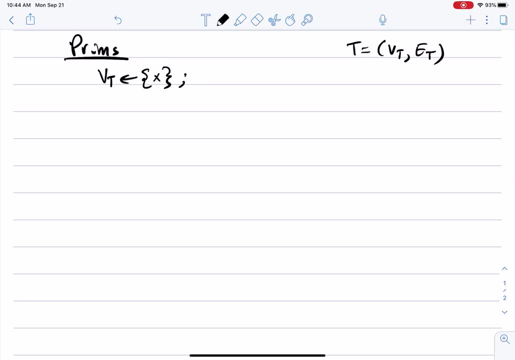 Arbitrary is not. I'm not talking about randomness here. I'm talking about: just take whichever node you want, the first one you encounter, And so this is the node from which we will start building the spanning tree, And the spanning tree now has no edges in it whatsoever. okay, 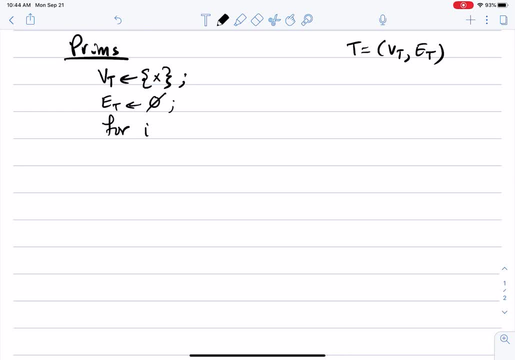 Then I will loop, for if that graph has n nodes, I will loop for n minus 1 times. okay, Why do I need to loop for n minus 1 times? Because if, If I have a spanning tree, I have a tree on n nodes, that tree will have n minus 1 edges. 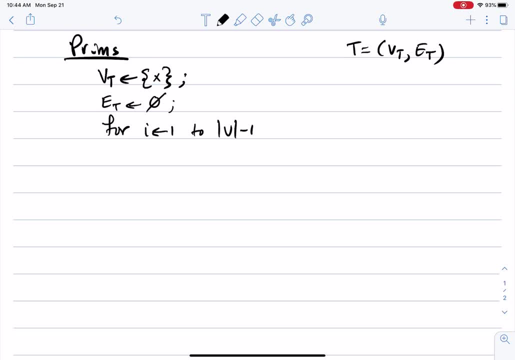 So I will loop the size of V minus 1 or n minus 1 times. Each time I will be adding one edge to the spanning tree. okay, By the time I added n minus 1 edges to the spanning tree, then I have a tree that spans to the entire graph. 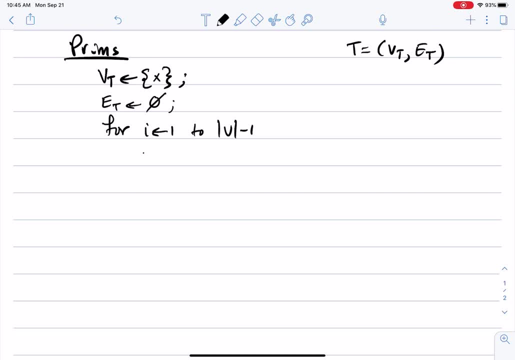 So then I will basically say: find the lightest- Or I shouldn't say the, because it could be multiple ones- Find a lightest edge. uv. e equals uv in the set e. set e of the edges of the graph. 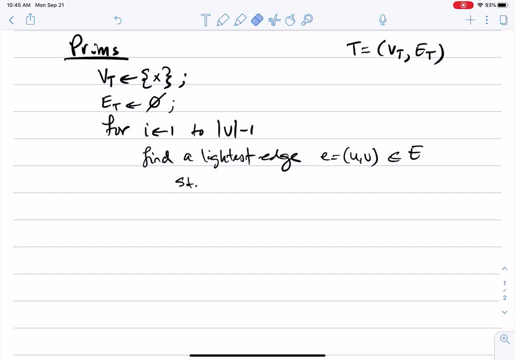 such that, such that we want to take that u, which is in v sub t, and v is in v minus v sub t. okay, What am I doing here? I want to find the lightest edge that connects the nodes that I have in v sub t. 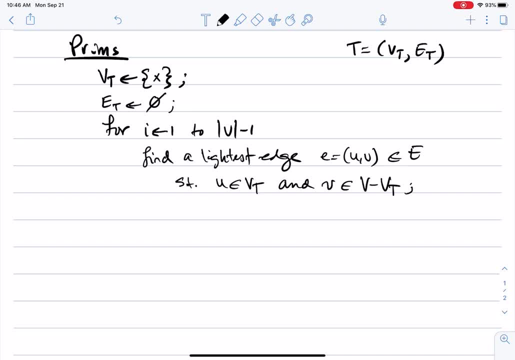 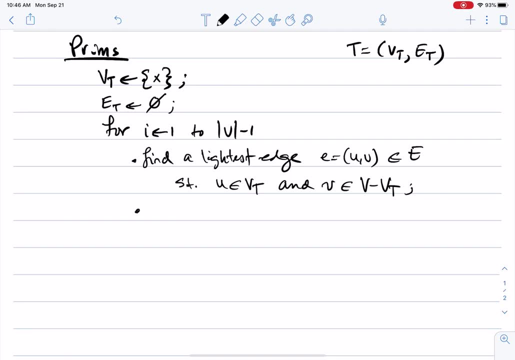 to the nodes that are outside v sub t. I will get back to this very quickly now, very soon, And basically, once you find this edge. now you can basically say v sub t. since u is in v sub t, I don't need to add it. 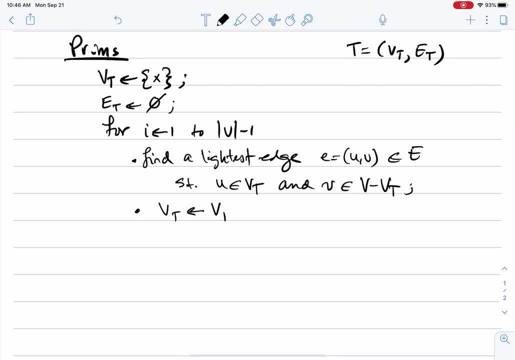 v is the new node that's not in v sub t. I can now add v sub t. I can add to it the node v And the e sub t is e sub t union, this new edge that I found- e, And then we basically return this pair v sub t, e sub t. 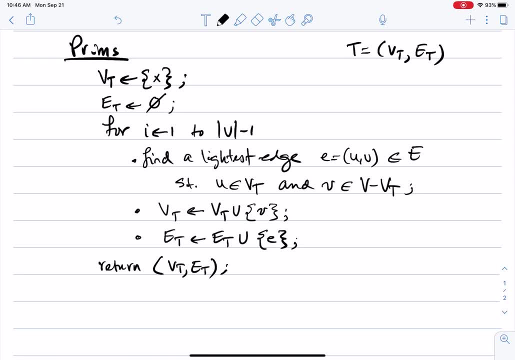 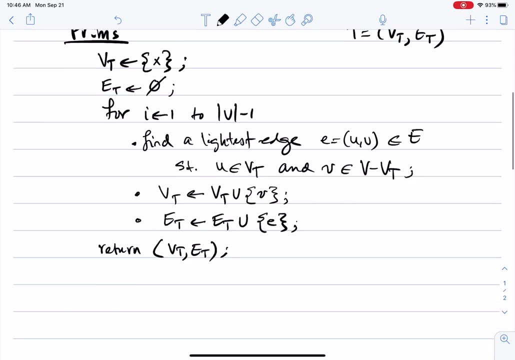 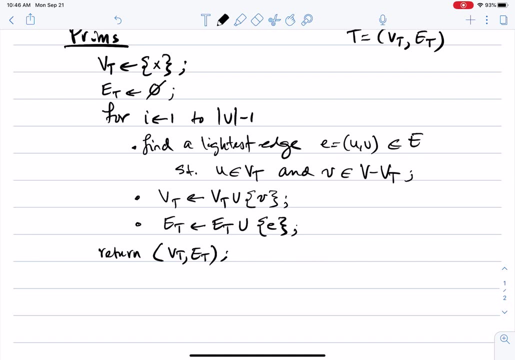 which is the minimum spanning tree. okay, So how is this algorithm working? okay, How is this algorithm working? It's very important to again, I need to scroll down so that the pseudocode will disappear. now, But again, think about it at. I am growing this set of nodes. v, sub t. 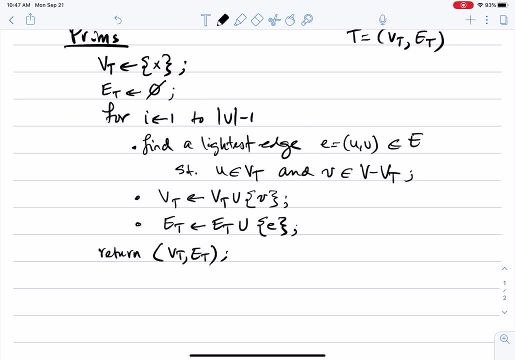 which will be then all the nodes in the spanning tree. At every point I look at a node, that at an edge, whose two endpoints, one is in v sub t and one is not in v sub t, And I add. I add it to the spanning tree. okay. 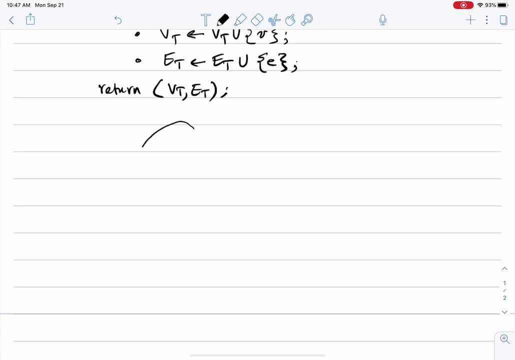 So, if you look at it at every point, at every point we have, If I have, this is here the subgraph that has v sub t in it and this is going to have the nodes v minus v sub t And what we are doing here. imagine that in v sub t here. 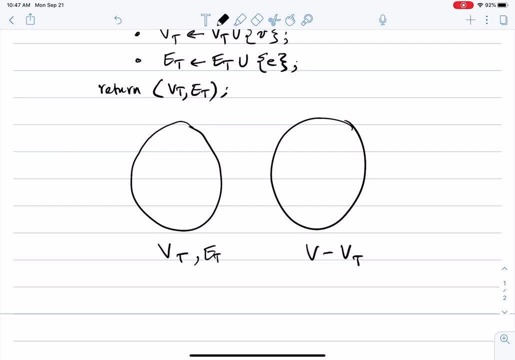 and e sub t as well, that I have the tree that I am building Now. okay, So imagine that I have this tree that I have been building And on v minus v sub t, there is the rest of the graph that has the node v minus v sub t. 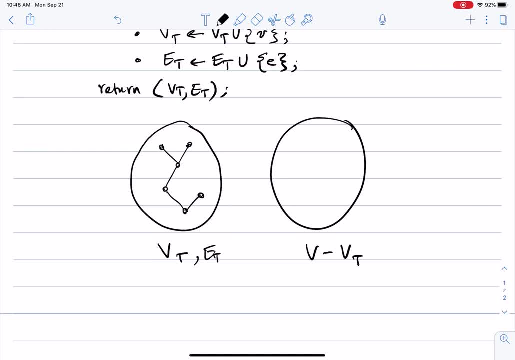 And the remaining part of the minimum spanning tree is somewhere there. okay, So imagine that this one still has, let's say, something like this, And this star here on the right, the five-node subgraph that it's. I will add it to the minimum spanning tree that I'm growing in a greedy manner. 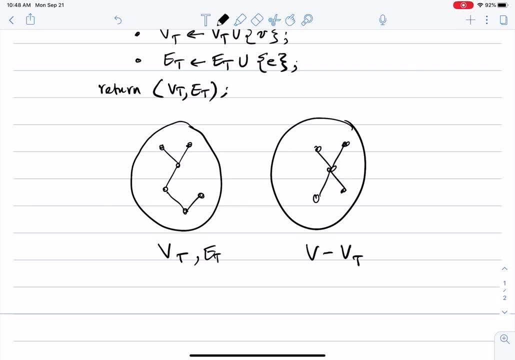 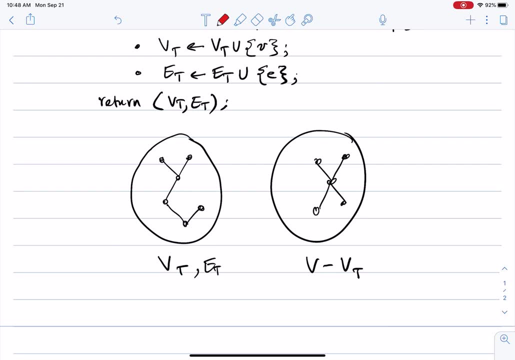 I'm adding it edge by edge. So what we are saying here is that look for that edge e. Look for that edge e that connects u and v, for example, something like this: So this will be the u and v And this will be the lightest. 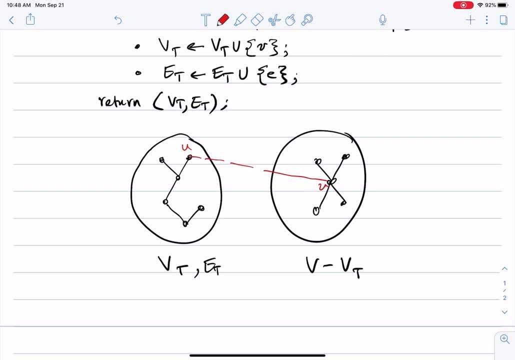 This will be the lightest edge of all possible edges that cross from the left to the right here. okay, So u is in v sub t and v is in v minus v sub t. It's very important that we chose it like this, because when I choose it like this, 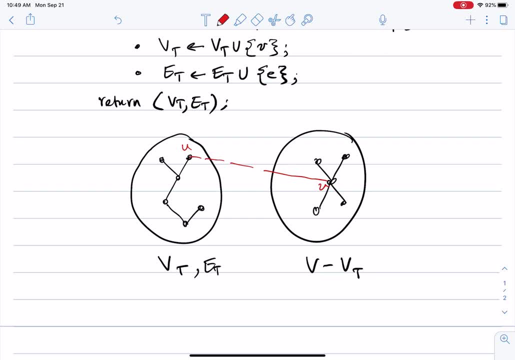 adding e to e sub t will not create a cycle, right? Because if I found the edge e equal uv to be an edge between two nodes in the same in here, I would have created a cycle, And this is bad, okay, So we don't want this. 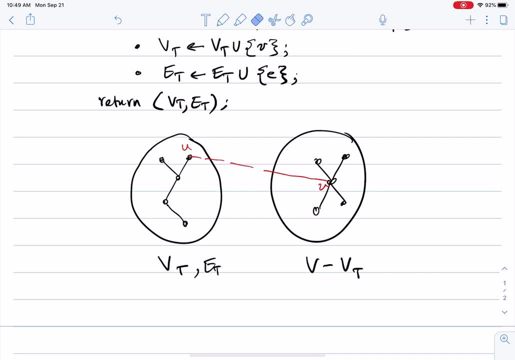 This is why the algorithm will always look for a node that is not in v sub t. okay, It's not in v sub t. So this is how the algorithm is going to work: by finding a node that is in v minus v sub t. 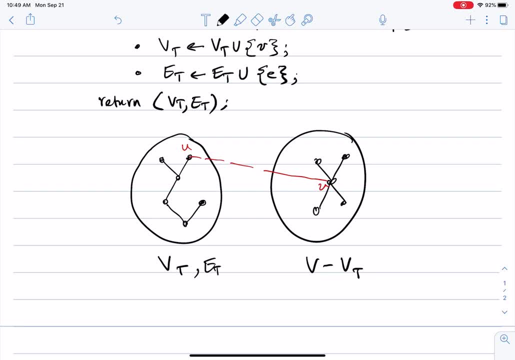 such that that edge that connects u to v, whatever u- okay, We are looping over all u's there in vt And this has the lightest edge. Now, why does this guarantee that the solution, the minimum spanning tree that Prim's algorithm is building? 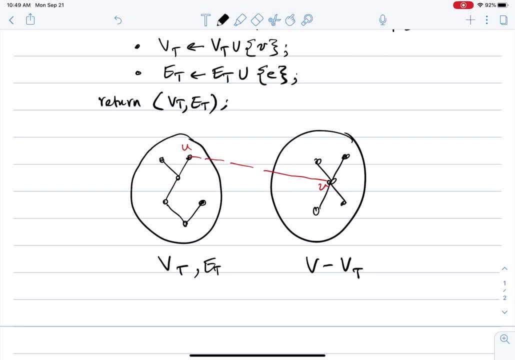 is optimal. So again we go back to the same proof technique and we say: let's assume it is not optimal. okay, So let's assume that this edge e, let's assume this edge e that the algorithm chose should not have been added. 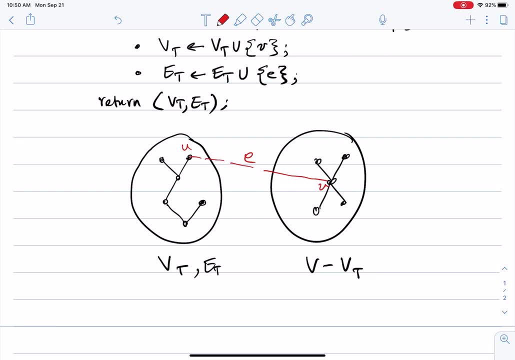 So again we go back to the same technique. Imagine that. let me label it by blue now. Imagine that this sub tree here both the Prim's algorithm and the optimal solution that is not Prim's algorithm- both agree on okay. So let me take it back one step. 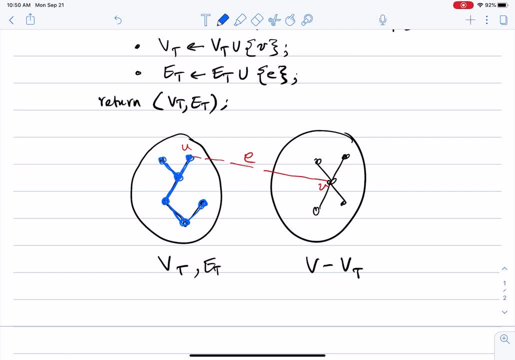 Prim's algorithm. we want to prove that Prim's algorithm is optimal. Proof is by contradiction: I will assume it is not optimal And then I will say that it's not optimal. It means that the minimum spanning tree or the spanning tree returned by Prim 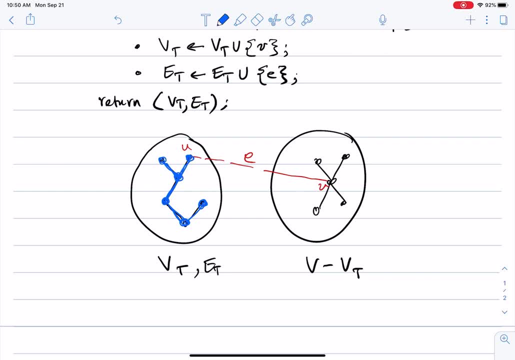 has heavier weight, has a weight larger than another spanning tree. okay, So let Prim's algorithm, the tree returned by Prim's algorithm and that other solution agree on this blue sub tree And in the next step, Prim's algorithm is going to choose e. 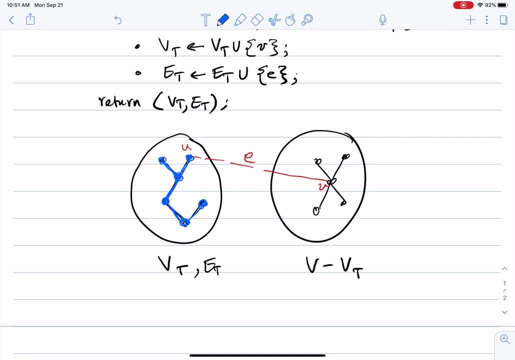 this red edge e, whereas that optimal solution will have a weight of e. So let's have another edge e, prime, okay, Something like this: okay, So again this. we go back to exactly the same technique, where we are saying: 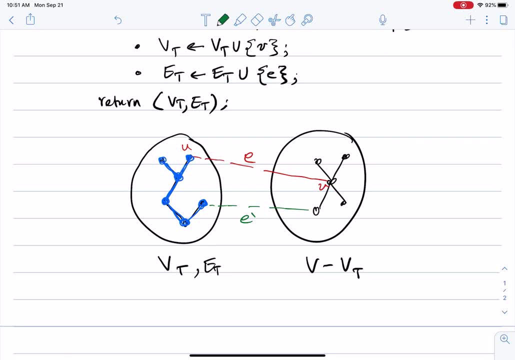 let e and e prime be the very first edge in which both the Prim's solution and the optimal solution disagree on. okay, Because remember that the greedy algorithm is building the solution step by step. So Prim's algorithm added the first edge, the second edge, the third, the fourth. 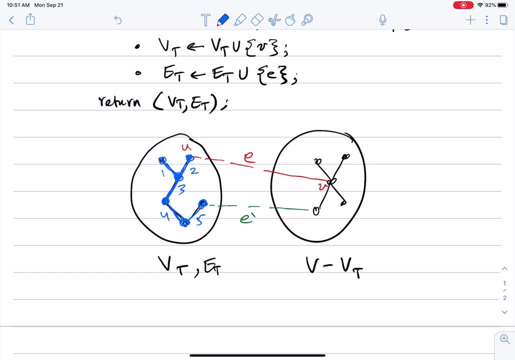 the fifth and these five edges agree between Prim's algorithm tree and the optimal solution that someone claims it exists and it's better than Prim's algorithm. So now let's focus on the next edge that Prim's algorithm will add, and let it be this red edge e. 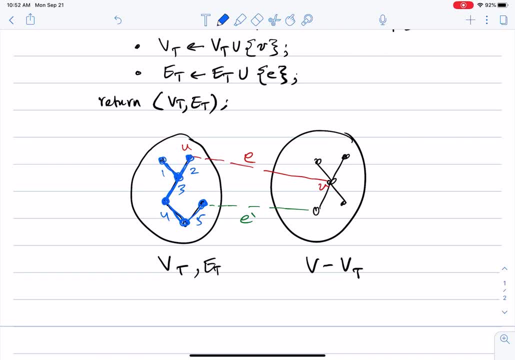 And we say: this is the first edge that is going to differ from that optimal solution, And in this case it's e prime. okay, So the optimal solution will have e prime, Prim's algorithm will have e. So now again, as we did before, 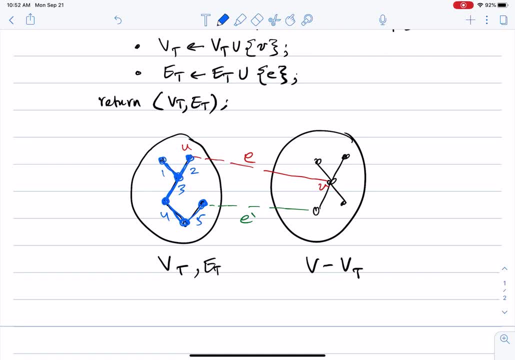 with the compatible intervals problem. we will see exactly the same issue here. e must have a weight that's smaller than e prime, because if e prime had smaller weight than e Prim's algorithm would have chosen e prime okay. So since e has lower weight, 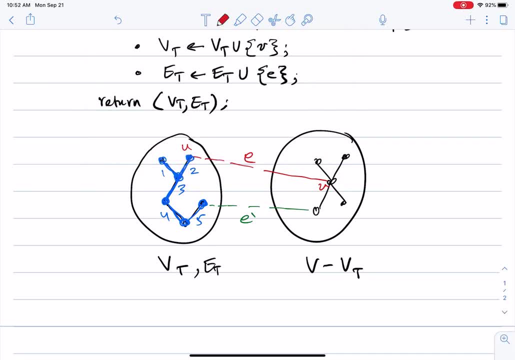 so I again, I will claim or make the statement here: w of e is smaller than w of e prime. okay, Of course, if it's equal, then we don't have even an argument here. okay, So e and e prime were the first two edges. 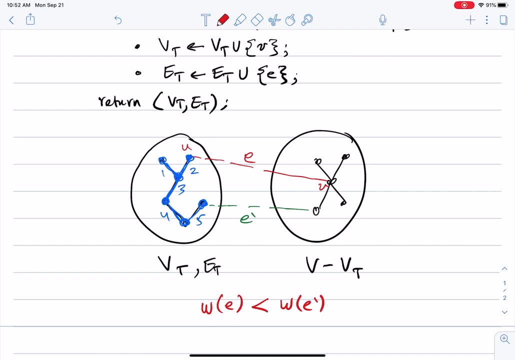 whose weights are different, and Prim's algorithm chose e and the optimal solution that we are assuming for the sake of contradiction has W of e. the weight of e must be smaller than the weight of e prime. If it wasn't, if the weight of e was larger. 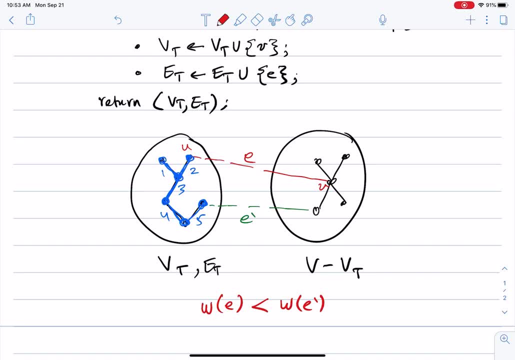 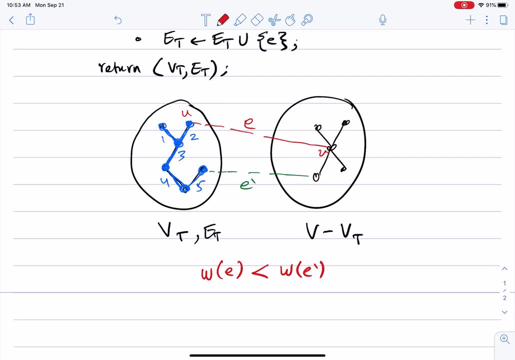 than the weight of e prime. Prim's algorithm would have chosen e prime. okay, So the weight of e is smaller than the weight of e prime. Now what is the weight of the minimum spanning tree Prim's algorithm? Prim's algorithm says that. 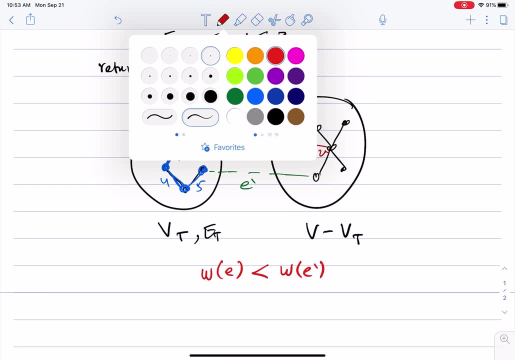 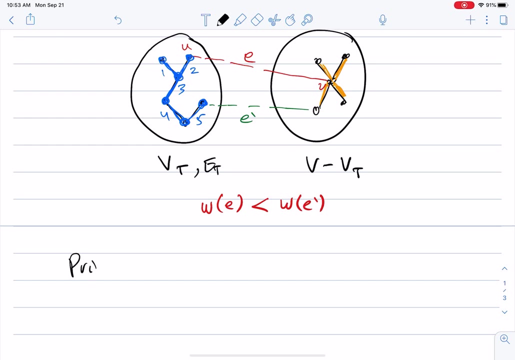 okay, let me actually color these ones here by orange. okay, So let me color these by orange. So, under Prim's algorithm, Prim's tree, Prim's tree, the weight of this is the weight of blue edges plus the weight of orange edges. 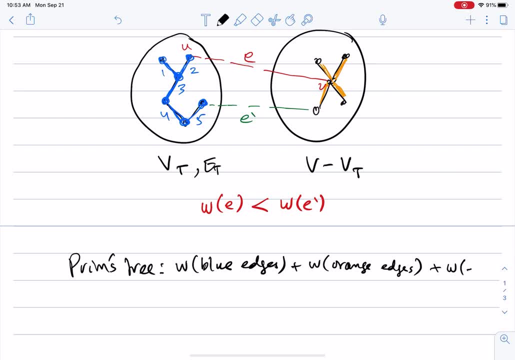 plus the weight of e, The optimal, the optimal tree that we are assuming. just for the sake of contradiction, its weight is the weight of the blue edges plus the weight of, for example, in this case, the weight of the orange edges. 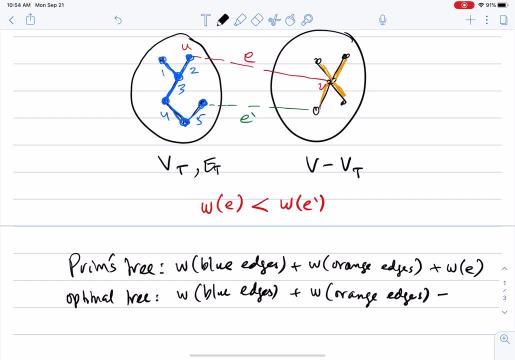 plus the weight of e prime. Okay, Now, if you think about this, the blue edges plus the blue edges plus the orange edges, plus e, plus e prime, it's almost as minimum spanning tree, or it's almost a spanning tree. 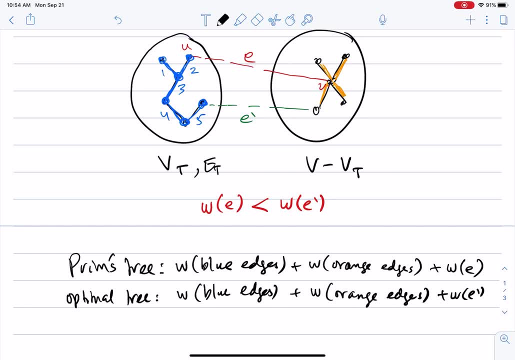 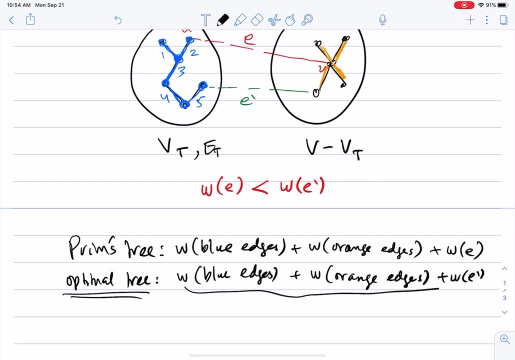 but we have a cycle Now. that cycle is caused because we have e and e prime. Now, if I look at this optimal solution, imagine that I subtract from it. I subtract from it. let me actually put it in a different color. 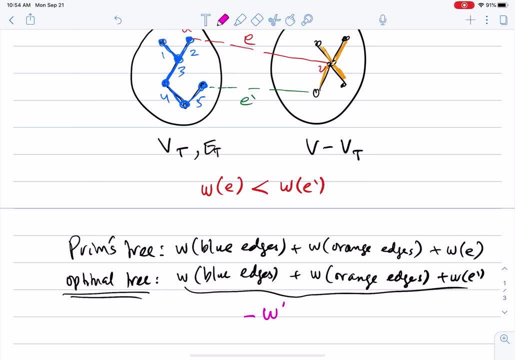 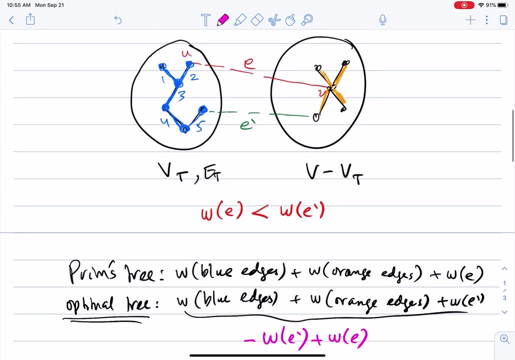 Imagine that now I subtract from it the weight of e prime, So I remove e prime but I add e. So if you remove e prime but add e, we have broken the solution. okay, we have broken the cycle and we replaced an edge e prime by another edge e whose weight is even. 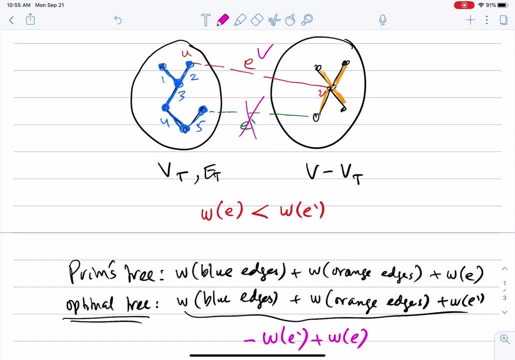 lower. so we cannot have e prime. we have. if we actually replace e prime by e, the only thing we can do is either keep the weight the same or even improve the weight of the solution. okay, so this is the. this finishes the proof. again, to recap the proof: assume that prim's algorithm is not optimal. 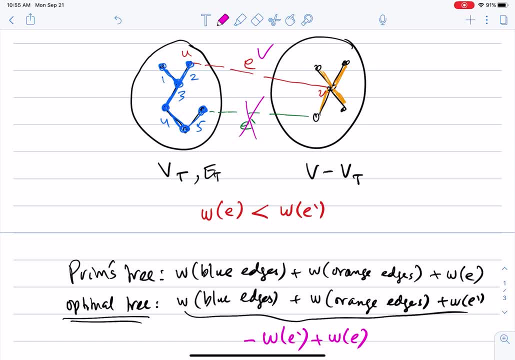 and that the algorithm that it gives us some tree and but there exists another tree whose weight is smaller than prim's tree. then i will say: let us look at the very first edges that prim's algorithm added and the very first edges that are in the other optimal solution in which both agree and let 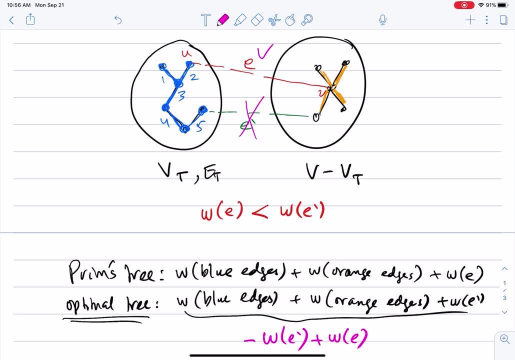 us focus on the very first edge that the, the algorithm and the optimal solution disagree on. these two edges are e and e prime. e is an edge that prim's algorithm decided to add, e. prime is an edge in the alternative, more optimal solution. and then how i proceeded to to show that this doesn't exist. 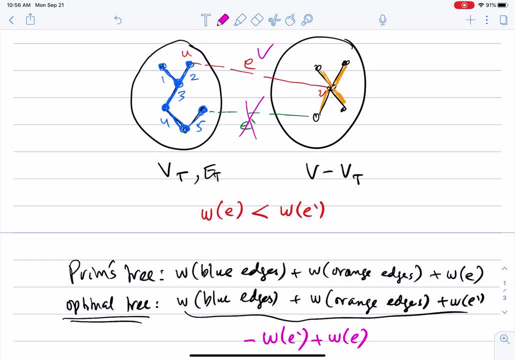 is by arguing that if i replace e prime by e, i still will have a tree. i will still have a spanning tree, and that new spanning tree that i created have even better weight than the original one. so i transformed now that optimal solution that someone claimed exists. i transformed it to be: 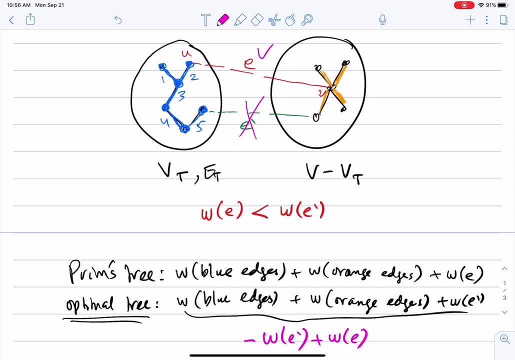 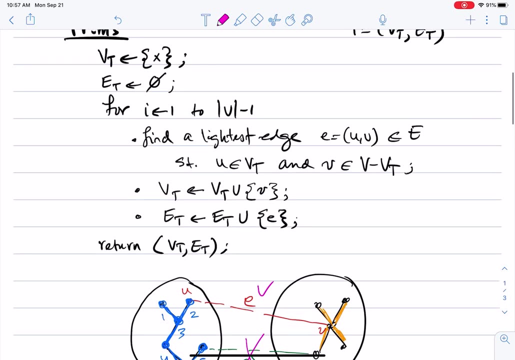 exactly the tree that was returned by prim's algorithm and without violating anything, without creating a cycle, still maintaining a spanning tree and only improving the weight of that. and this completes the proof of of prim's algorithm. now, if we go back, i want to go back to the pseudocode just for a second and look at the running time of this algorithm. the running. 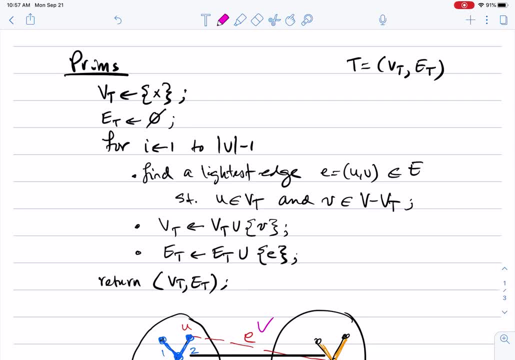 time of this algorithm, if we look at it. you know, this one here is: these: two are o of one right, and then we need to to look at the the loop here. so we need now to do this- does in iteration. so if the size of v is n, so we have n iteration. 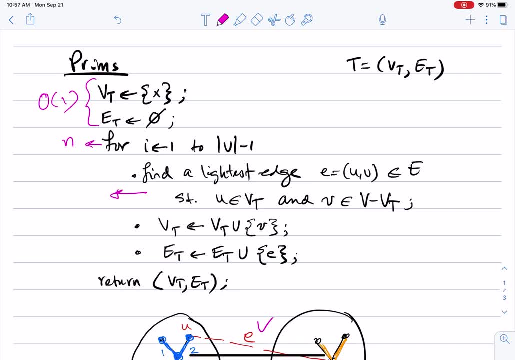 every time we need to find the lightest edge, and then we need to add it, and so on. now we use a min heap, which is a binary search tree that maintains the minimum element at the root, and finding the smallest element is o of one. but this is not o of one. here i cannot say o of one. 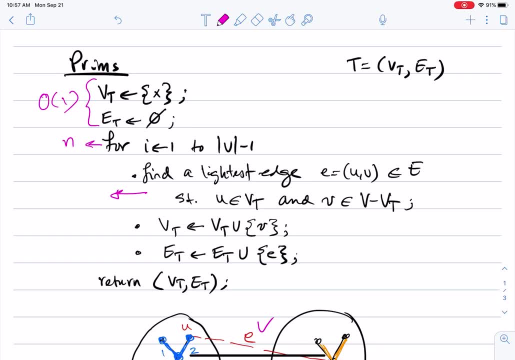 the reason for this is because i am maintaining in a heap, the, a heap of size n, the nodes, the nodes v and v minus vt, in terms of their distance to that set v sub t. okay, so we have a minimum heap that maintains that has the same number of nodes as the number in v minus v sub t. so if we still 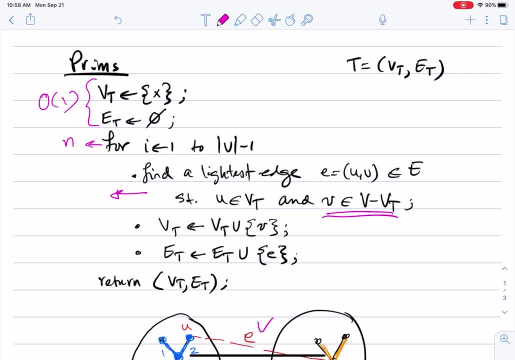 have 15 nodes in v minus v sub t, we will have a minimum heap with 15 nodes in it for every node. there, at the top of that heap we have that node v, whose edge that connects v to a node in vt. it has the smallest weight. 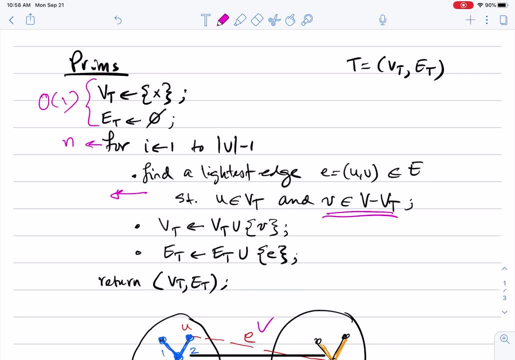 so that next time we choose it now, when we use that u equal uv, e equal uv and we add v to v sub t, now we have to update the heap, okay, so this is why this ends up being o of log n, because we need to find the lightest edge, and then we need to update the heap there, and these are o of one. 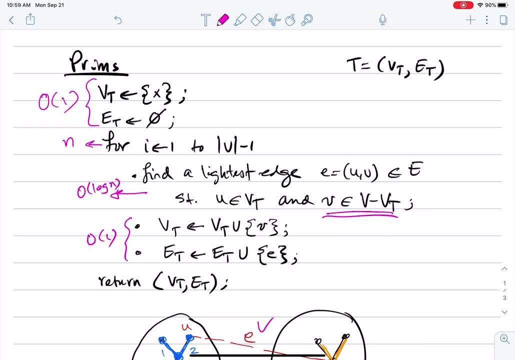 here in. in some sense we just need to add the edges and the nodes and the number, sorry, the num. the this o of log n is the time it will take to update to up to, to make one update to one node, but this this o of log n end up being done. 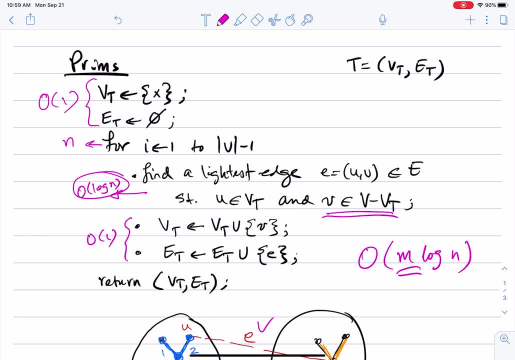 m times. okay, so if m is the number of edges, we have to update it m times, because with every edge e that we inspect or we add, we have to update this. okay, so the the details of the running time. actually you can find them written in the, in, i'm sure, in clrs or in any other algorithms book. 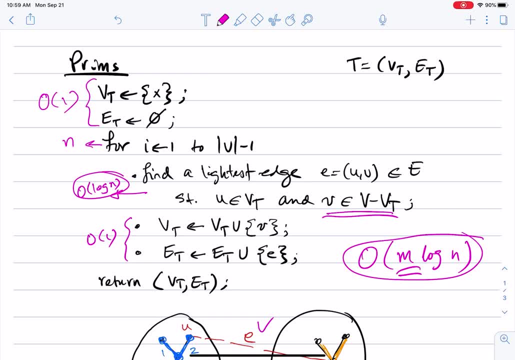 you should look at them, because using the heap is what gives us the o of m log n. if you don't use the heap and if you assume adjacency matrix, you will get to some running time that is quadratic. but if you use a heap to represent the nodes in v minus v sub t, in v minus v sub t, then updating. 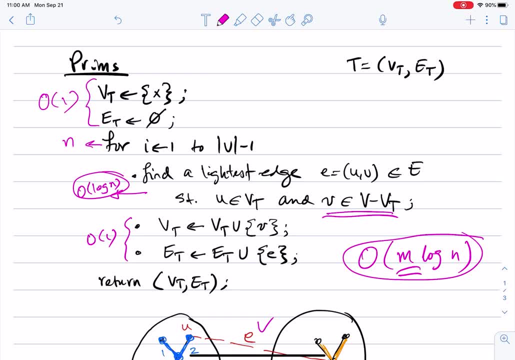 is in in that heap is o of log n. but the number of updates we we end up doing is on the in the worst case is as a number of edges in the original graph. so the running time of the prim's algorithm is o of m log n. okay, there could be the n log n factor there, but since i'm assuming the graph 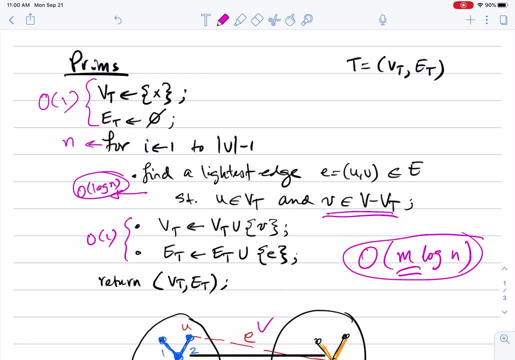 is is connected. m is always larger than n, or m is larger than or equal to n. okay, so prim's algorithm is a polynomial, is a is a logarithmic algorithm, it's m log n. it is correct as we showed. the proof is again the same technique as we show for the. for the compatible intervals problem, you first assume the algorithm. 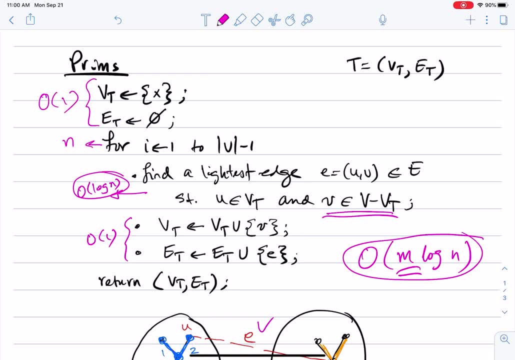 is incorrect. you focus on the, the sub solution, the for the prefix of the solution on which prim's algorithm and the other optimal solution agree on. focus on the first edge they disagree on, and try and and replace the edge in the optimal solution by the edge that prim's algorithm found, and you will find that you can only improve that. 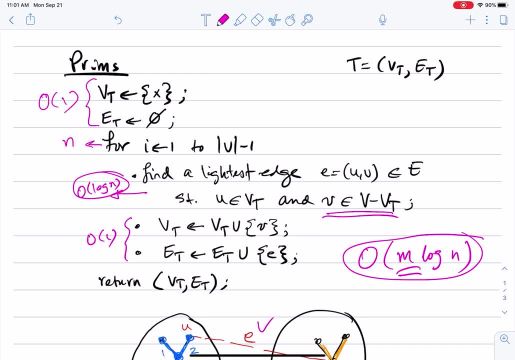 so why not even take it from the the beginning, which is the contradiction, that there is an, a solution that's better than prim's algorithm?